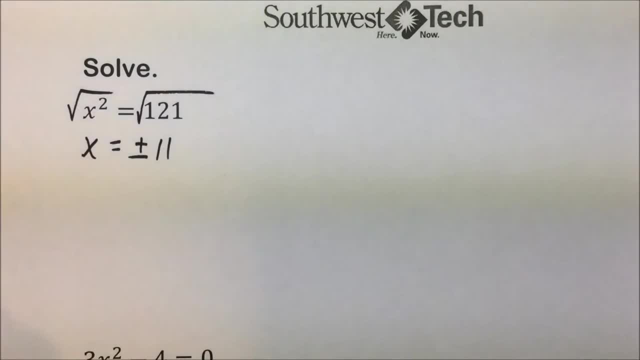 minus And in this case square root of 121 is 11.. We can separate this into x is equal to 11 or x is equal to negative 11, using the principles of square roots. In this next problem it's not quite of that generic form of something squared equal to a. 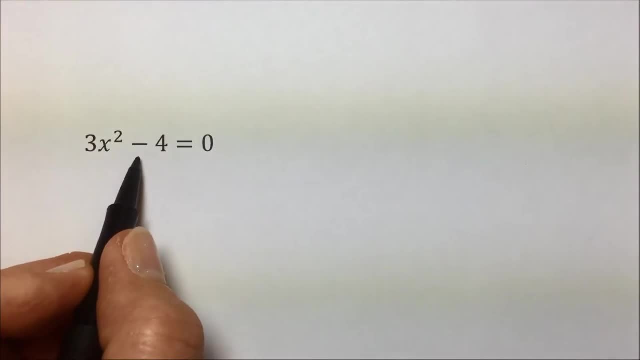 number. but if we solve for the variable by adding 4 to both sides, leaving us with 3x squared is equal to 4.. Furthermore, dividing both sides by 3 leaves us with x, squared is equal to 4 thirds. 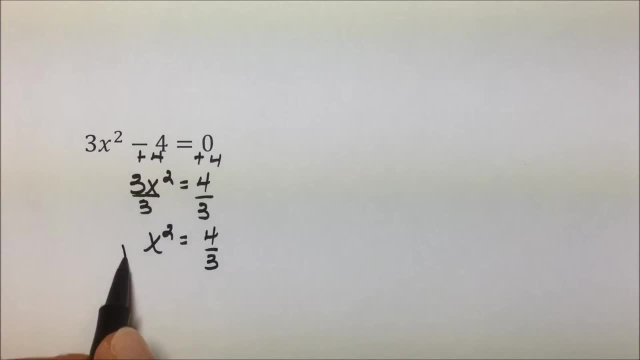 We now can use the principle of square roots, taking the square root of each side. square root of x. squared is x. it will equal the positive version for the square root of 4 thirds, as well as the negative version of the square root of x. 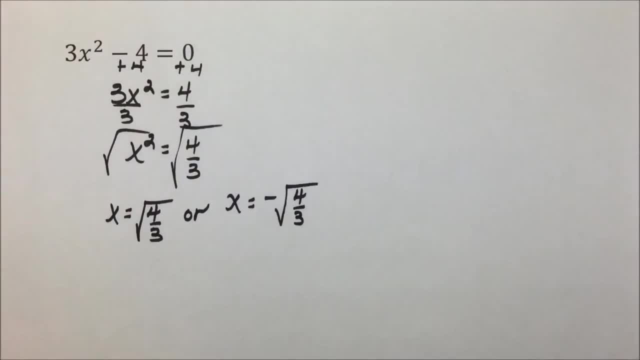 4. thirds, Simplifying our solution here, we can take the square root of the numerator, which is 2, over the square root of the denominator. likewise on the other one, and while we're at it, rationalizing the denominator by multiplying top and bottom by the square root of 3. 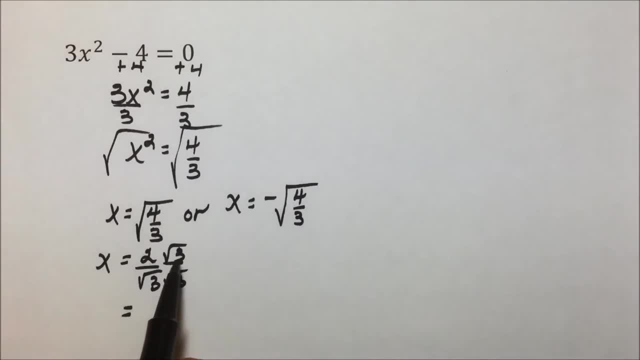 our best form of our answer would be a positive: 2 square root of 3 over square root of 3 times square root of 3 is 3 and of course, this term also would simplify into the negative version of that: 2 times the square root of 3 over 3. 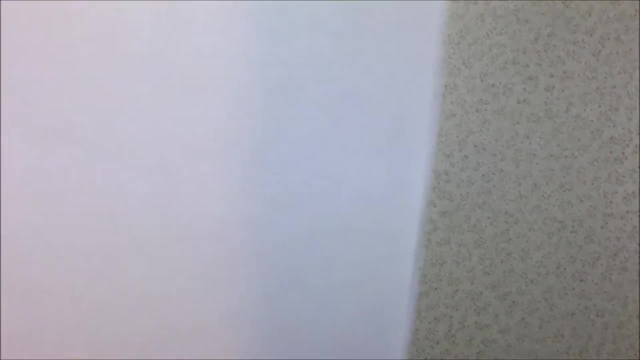 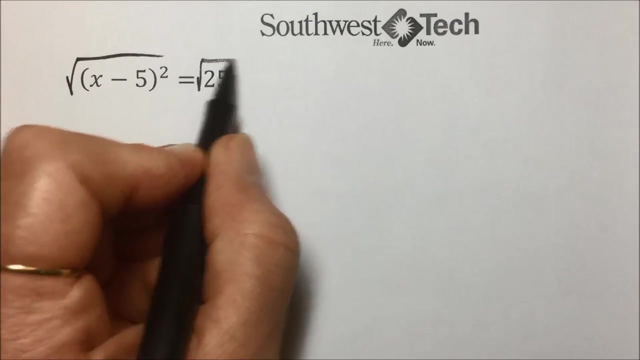 Adding a little more complexity, but still of the same form of something squared is equal to 25, we can use the principal square roots here as well. The square root of this quantity, as well as on the right, will give us the radicand x minus 5. 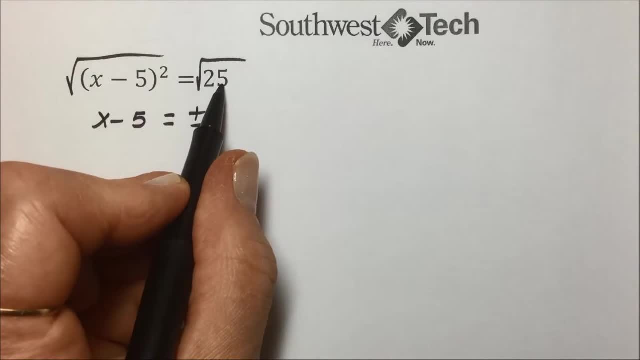 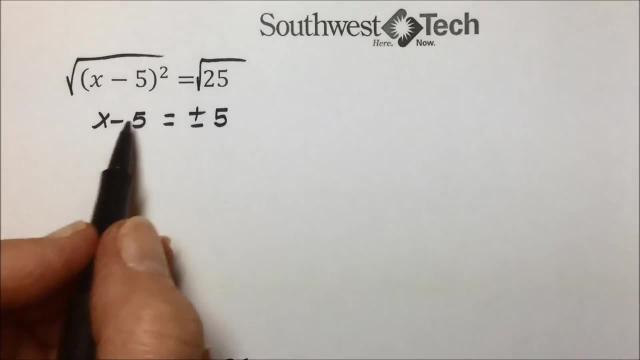 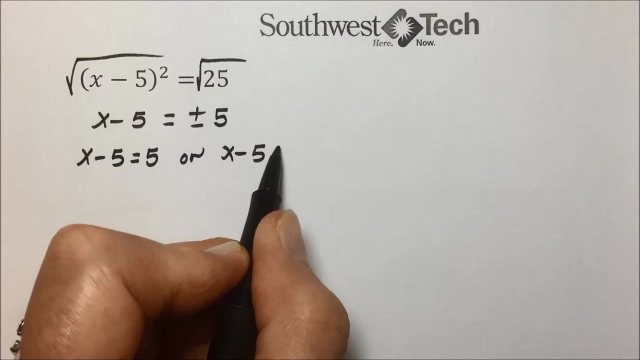 and it will equal the positive root of 25 and the negative root of 25, which in this case is 5.. Separating these, then we have: x minus 5 is equal to 5, or x minus 5 equals negative 5. Solving this equation. 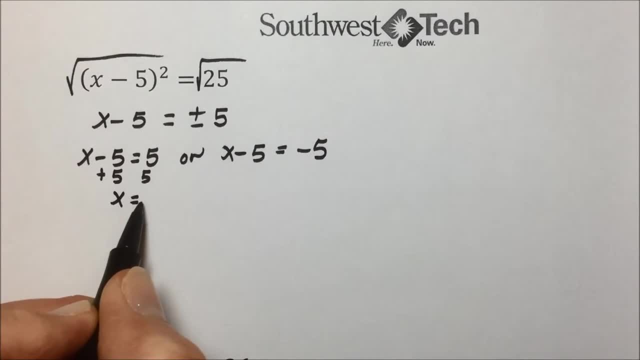 we'll add a 5 to both sides, we end up with x is equal to 10.. Solving here: adding a 5 to both sides, we end up with x is equal to 0. So our solution for this problem is 10 or 0, and we can plug that in to verify that it does work. 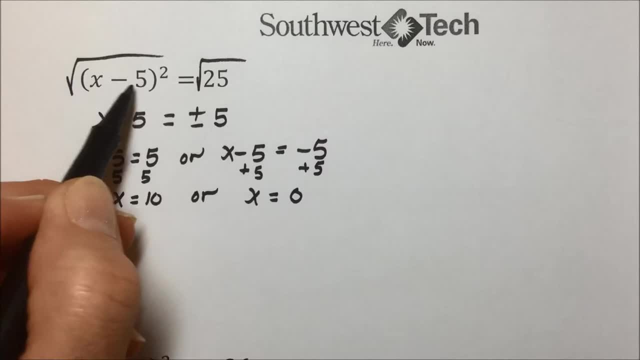 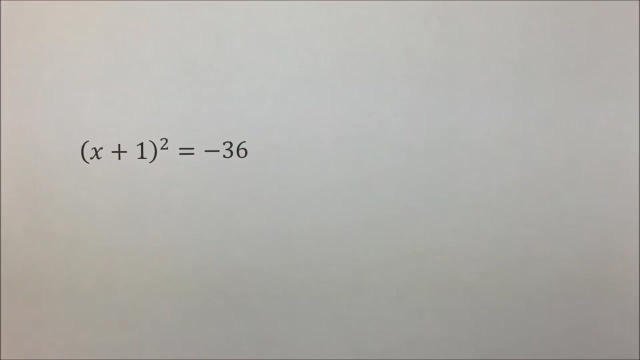 10 into the original equation for x would give us a 10 minus 5, which is 5.. 5 squared would equal 25, and with a 0, 0 minus 5 squared would be a positive 25 as well. In this next problem, it looks a lot similar to the last one. 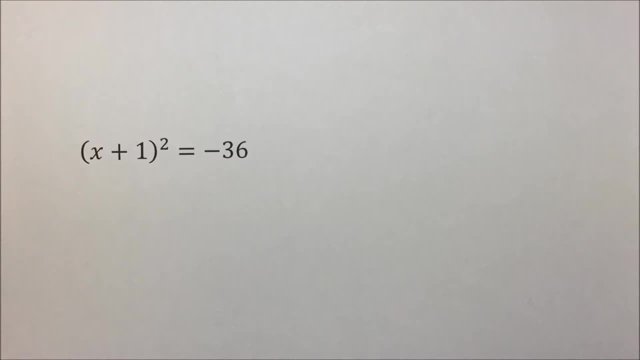 The principals of square roots apply, whether it's the real number system or the complex number system. so when we take the square root of each side to get down to our variable, in this case the square root of this quantity squared will be: the radicand is equal to the square root of 25.. 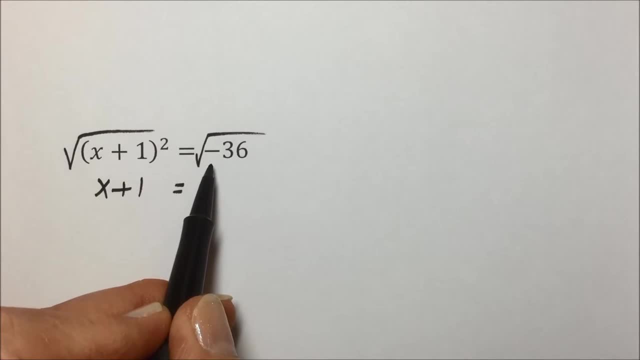 negative 36,. we can't take the square root of a negative number under the real number system. but we can replace that with the square root of negative 1 times the square root of 36, and use the complex number system to solve this. We will get. 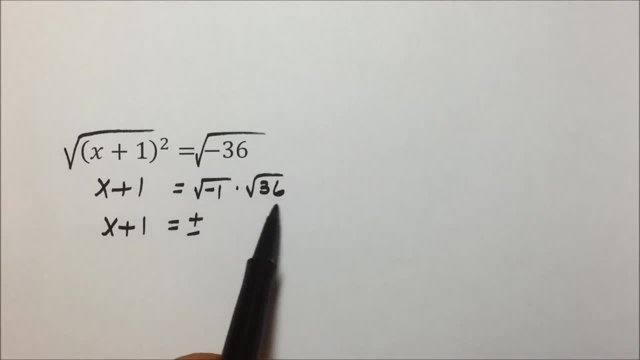 both versions, positive and negative, and putting our real number first, square root of 36 would be 6,, followed by the square root of negative 1, which we'll replace with an i. So our solutions will be: x plus 1 is equal to a positive 6i, or x plus 1 will. 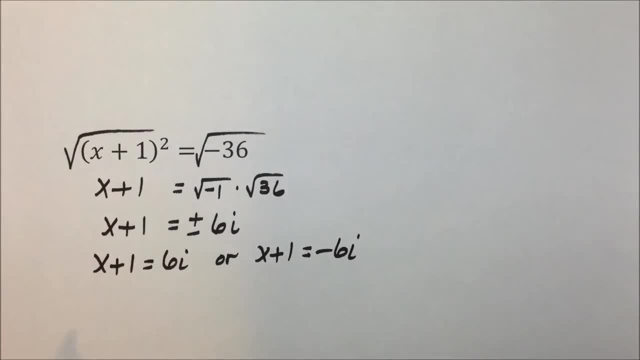 equal a negative 6i, Simplifying for the variable subtracting a 1 from each side. it's not similar with the complex, pure imaginary term here, so we'll end up with negative 1 plus 6i, the complex number subtracting. 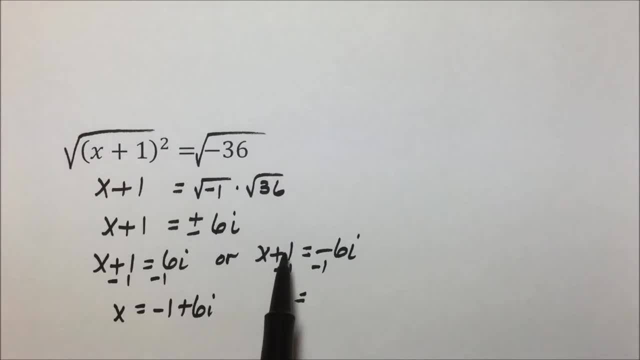 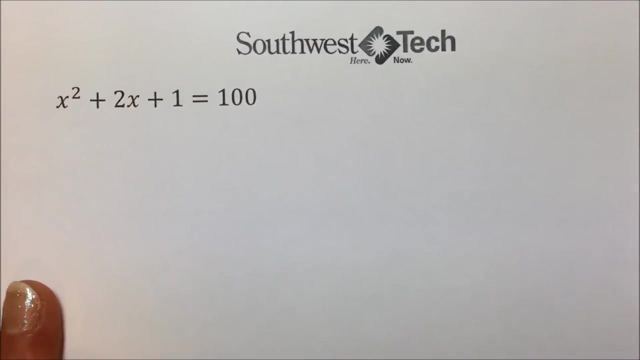 a 1, subtracting a 1 again for our other solution. These are not similar terms. We have a second complex solution for this equation. It's nice when the problems are already as perfect squares, but if they don't, and you do, recognize it as a perfect square, factoring.